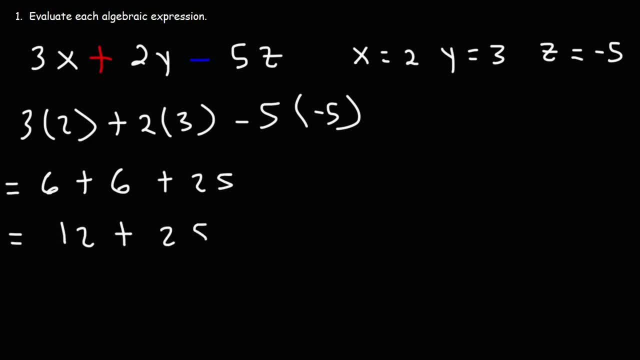 6 plus 6 is 12.. 12 plus 25 is 37.. So that's the answer for this first example. Now let's try another one. So let's say we have the algebraic expression x squared whoops plus 3x minus 4.. 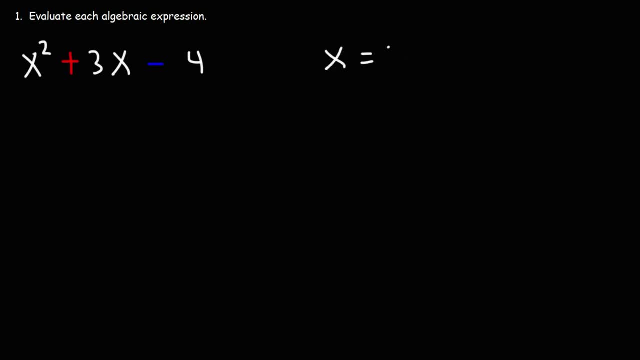 And let's say we're given that x is equal to 4.. Go ahead and evaluate the algebraic expression. So let's say we have the algebraic expression when x is 4.. So this is going to equal 4 squared plus 3 times 4 minus 4.. 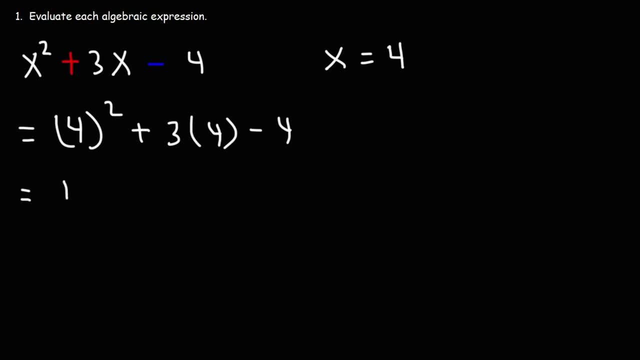 4 squared, that's 4 times 4, which is 16.. 3 times 4 is 12.. And 16 plus 12 is 28.. 28 minus 4 is 24.. So that's the answer. 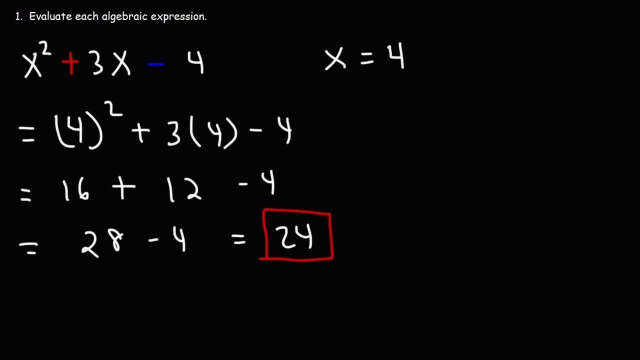 So that's the answer for the second example. Now let's work on some other examples. Consider this expression: 2x squared minus 5y plus 3. And let's say that x is 2. And y is equal to 3.. 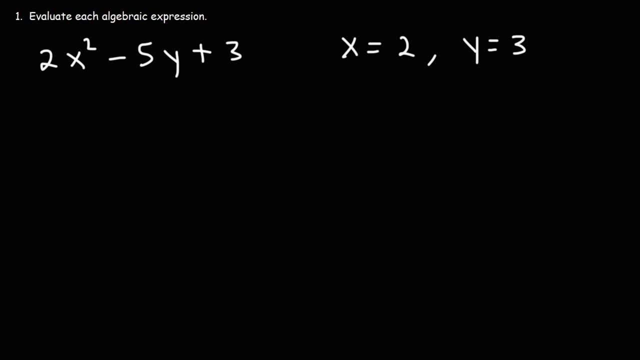 Go ahead and evaluate those expressions, given the values shown on the right. So we need to substitute x with 2. And we need to replace y with 3.. Now we need to follow the rules of whenever we're doing. order of operations. 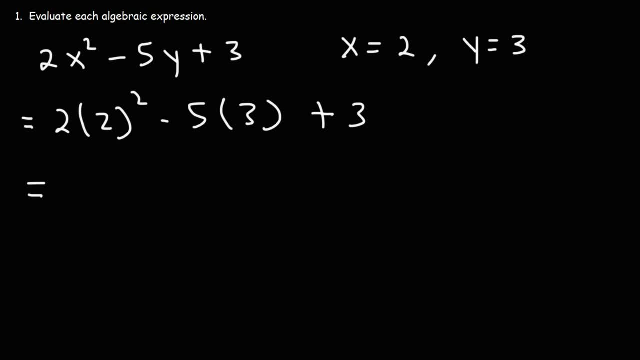 Which is, we should start with exponents. 2 squared is 2 times 2,, which is 4.. And 5 times 3 is 13.. Actually, no, 5 times 3 is not 13.. 5 times 3 is 15.. 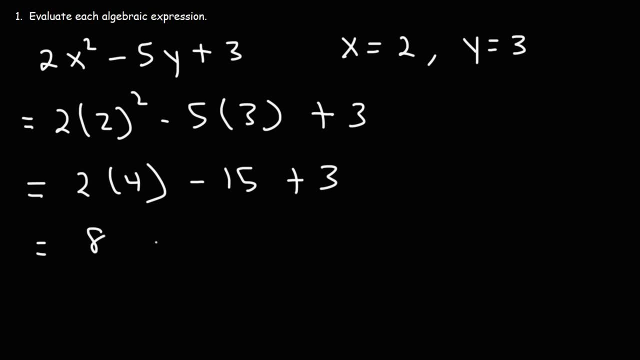 2 times 4 is 8.. Negative 15 plus 3,, that's negative 12.. And 8 minus 12 is negative 4.. So this is the answer. Now, if you ever want to check your work, I recommend plugging in what you have after you substituted x and y into a calculator. 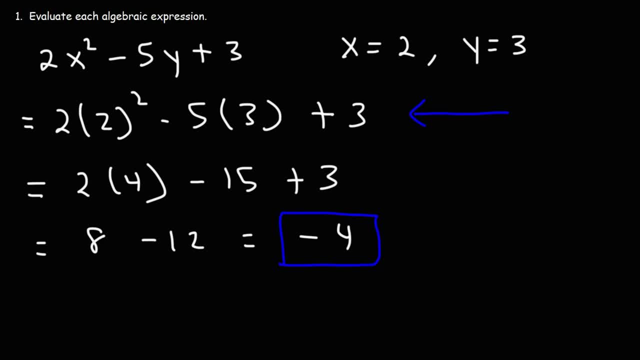 So if you take your calculator and type in 2 times 2 squared, and then minus 5 times 3 plus 3.. Check to make sure that it gives you your final answer, Which in this case it does. Here's another problem. 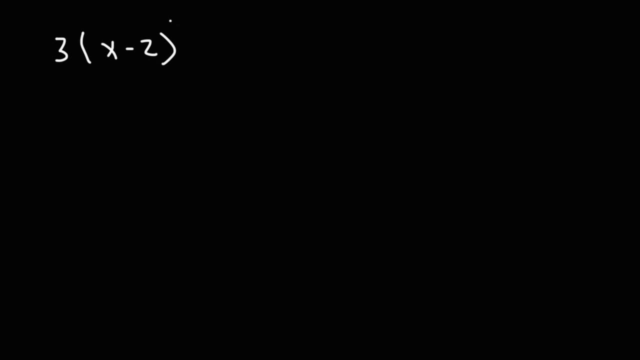 3 times x minus 2, squared plus 5.. And let's say that x is 6.. Feel free to try that example. So first let's replace x with 6., And so we have 6.. And so we have that. 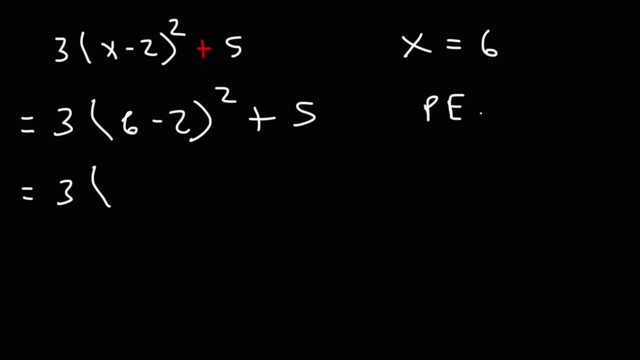 Now, perhaps you heard of the expression PEMDAS. Please excuse my dear and Sally, But when you see this expression, what it means is that we should work with the operations inside the parentheses And then we can work on the exponents. 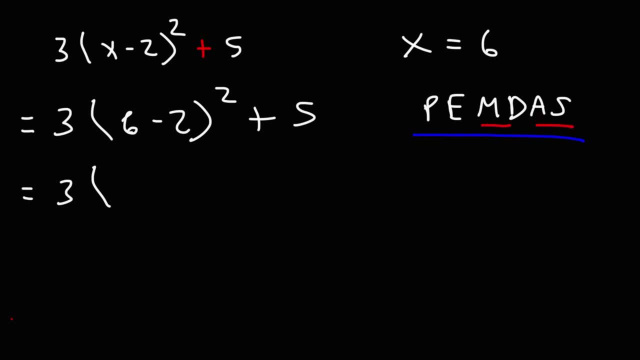 a and s means addition and subtraction, m and d means multiplication and division. The priority starts from the left and goes towards the right, So we need to work with the things inside the parentheses and the exponents first Before we multiply or before we deal with addition or subtraction. 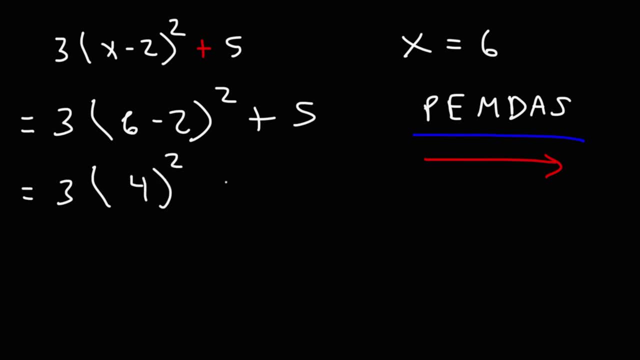 6 minus 2 is 4.. 4 squared, or 4 times 4, that's 16.. Now we won't add 16 plus 5.. We shouldn't perform addition. We need to perform multiplication first. 3 times 16 is 48.. 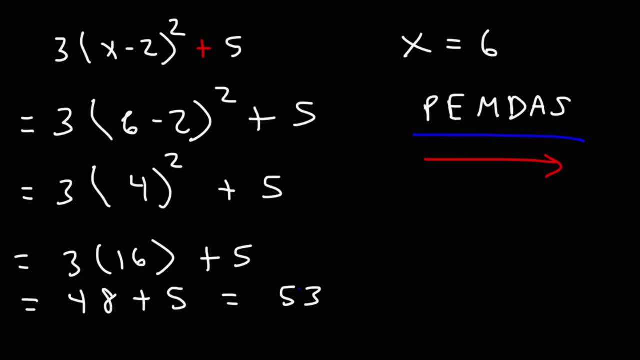 And 48 plus 5 is 53. So that's going to be the answer for this problem And if you want to check your work, simply plug this in to a calculator, Which I'm going to do to make sure I didn't make any mistakes. 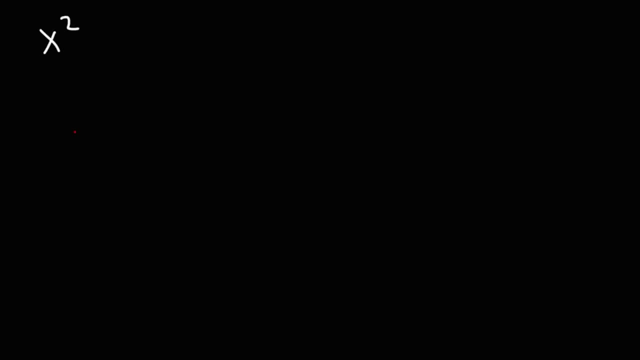 Here's another problem that you could try. Let's say we have x squared minus 5 times x minus y, raised to the third power, And let's say that x is 6, y is 3.. Go ahead and try that. So this is going to be. 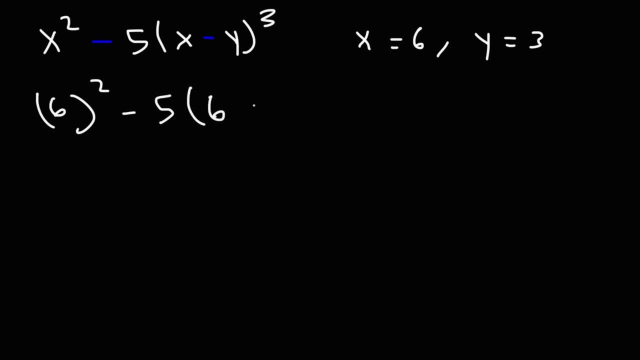 6 squared minus 5 times 6 minus 3, raised to the third power, 6 squared or 6 times 6, that's going to be 36.. Now, before we use the exponent, we need to work the operation inside the parentheses. 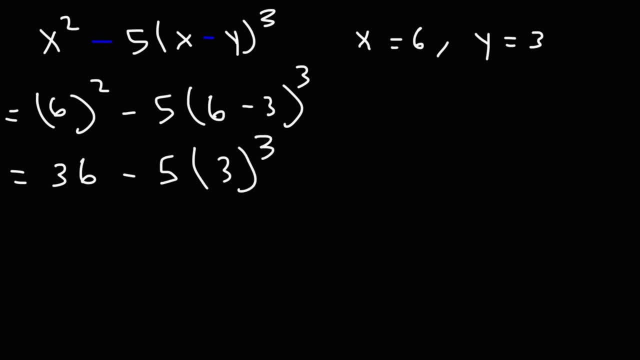 So 6 minus 3 is 3.. Before we subtract we need to work with the exponents first, And before we multiply we need to work with the exponents first. 3 to the third power, that's 3 times 3 times 3.. 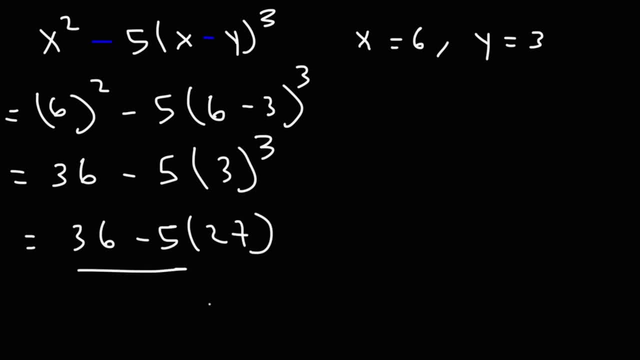 Which is 27.. Now, before we subtract, we need to multiply 5 and 27.. 5 times 27 is 135. And 36 minus 135.. The final answer? The final answer is negative 99.. But now let's make sure. 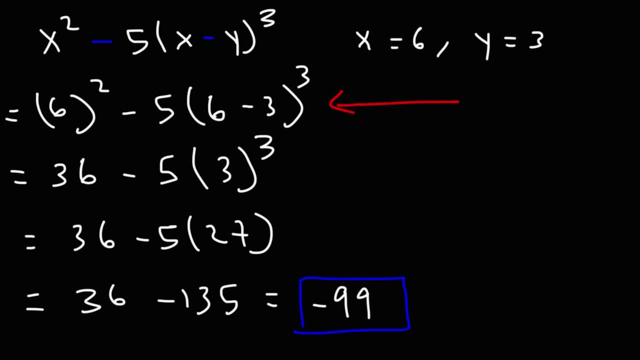 Go ahead and plug exactly what you see into your calculator, And this answer is indeed correct. So now let's move on to the next example. Let's say we have the expression x squared, And we're going to multiply, And we're going to multiply. 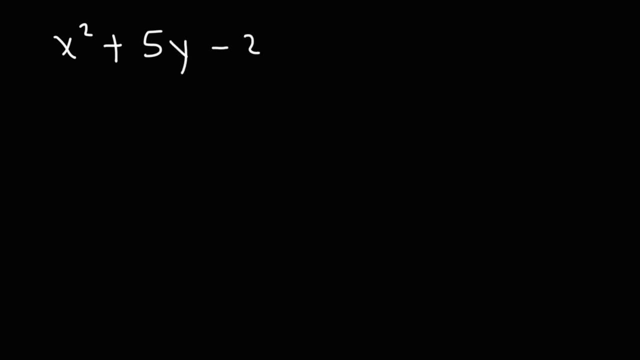 Plus 5y Minus 2xy squared, And let's say that x is 5, y is 4.. Go ahead and try that. So we're going to have 5 squared plus 5 times y or 5 times 4.. 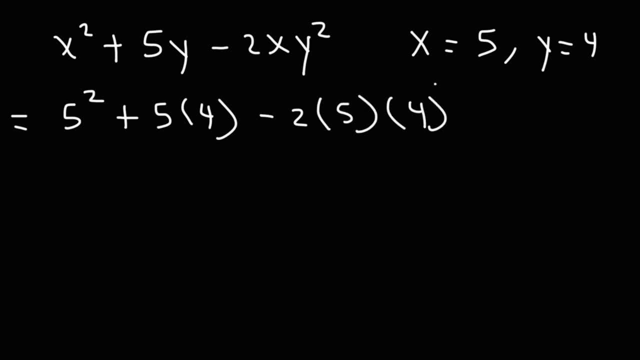 Minus 2x, and then y squared 5. squared 5 times 5, that's 25.. 5 times 4 is 20, 2 times 5 is 10 and 4 squared is 16. now 25 plus 20. 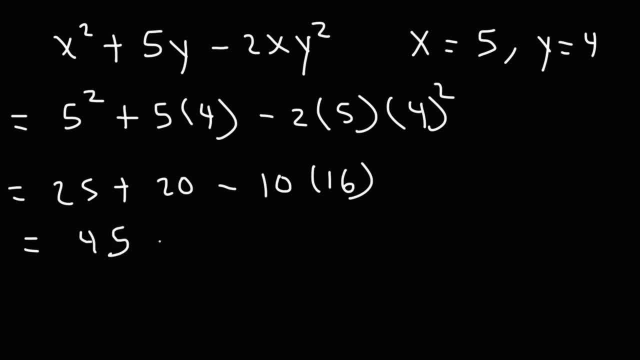 it's going to be 45, and 10 times 16 is 160. 45 minus 160 is negative 115. so that's the answer for this problem. but go ahead and plug everything in to make sure we have it right. that's how you know if you did it correctly. 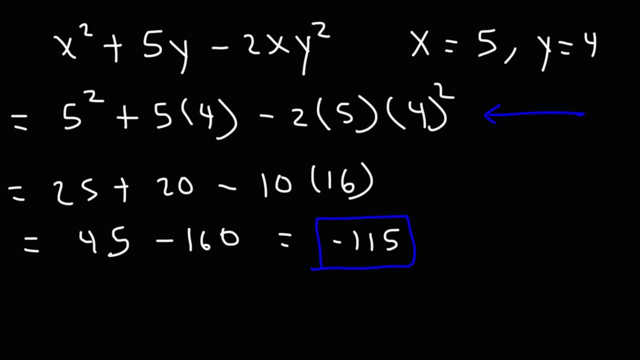 just plug in what you have after you substituted x and y into your calculator and see if it gives you the same final result which in this case it does. now let's say we have this: 3 times x plus 4 divided by x plus 4. 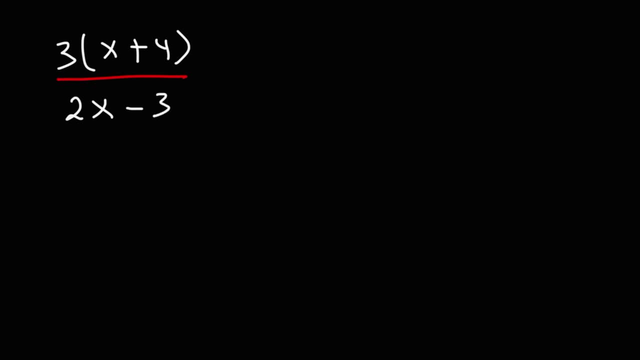 2x minus 3y. now let's say that x is 5, y is 2. go ahead and try that. so, replacing x with 5, we have 3 times 5 plus 4 over 2 times 5 minus 3 times 2. 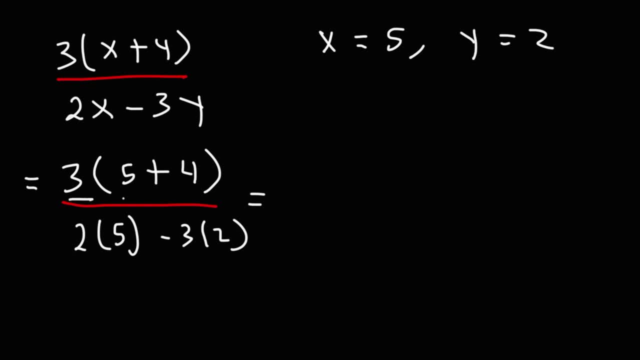 now, before we multiply, let's work through this and see if we can get the operation inside the parenthesis. 5 plus 4 is 9, and on the bottom we have 2 times 5, which is 10, minus 3 times 2, which is 6. 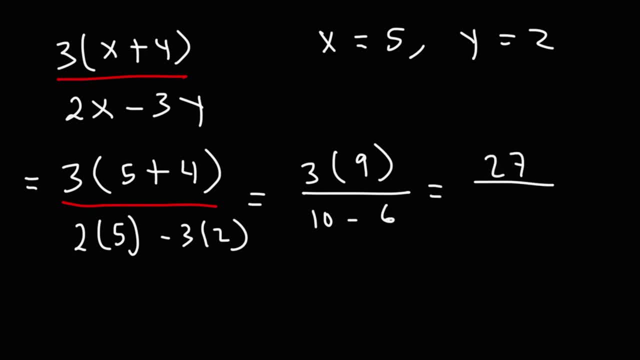 now, 3 times 9 is 27, 10 minus 6 is 4. so we can't really simplify this fraction, so we can leave the answer like this. but if we want to, we can get the decimal value of this. so we can get the decimal value of this. 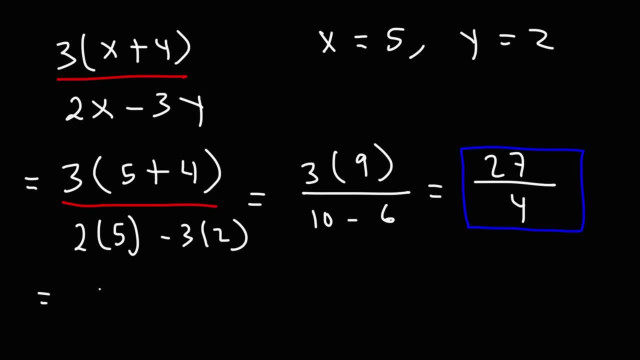 27 can be broken down into 24 plus 3, so 27 over 4. we can write it as 24 over 4 plus 3 over 4, because 24 plus 3 is 27. the reason why I broke it down like this: 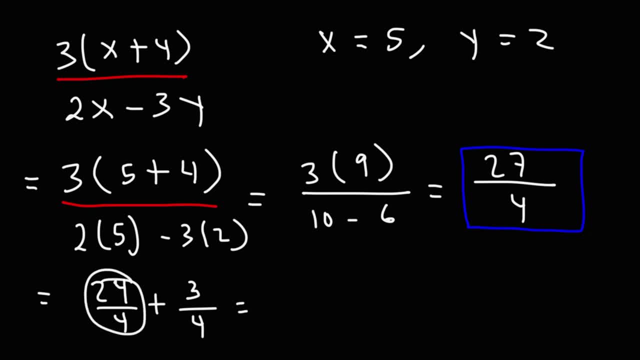 is because 24 is the highest multiple of 4, just under 27. 4 can go into 24, nice, and evenly, 24 over 4 divided by 4 is 6, so we have 6 and 3 fourths. so you could write your answer. 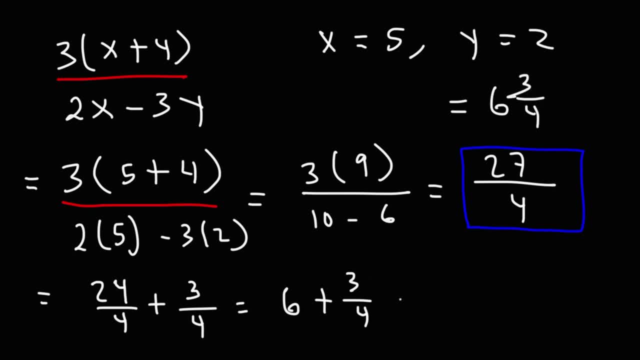 as a mixed fraction or you can get a decimal value of it. 3 fourths is the same as 3 times 1 fourth, and a fourth of something is 25% or 0.25, so this becomes 6 plus 3 times 0.25. 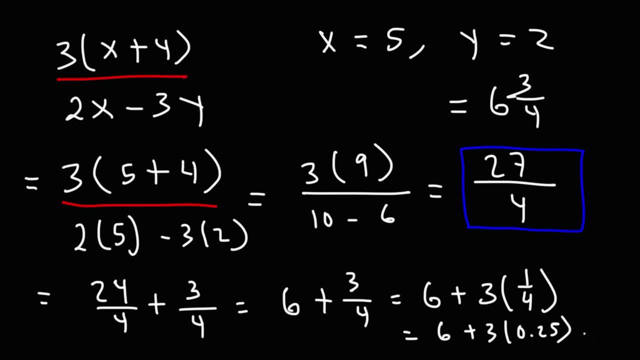 and 3 times 0.25, that's 0.75, so you get 6.75. if you want the decimal answer, so you can write your answer in any one of these three formats. you can leave it as an improper fraction: 27 over 4. 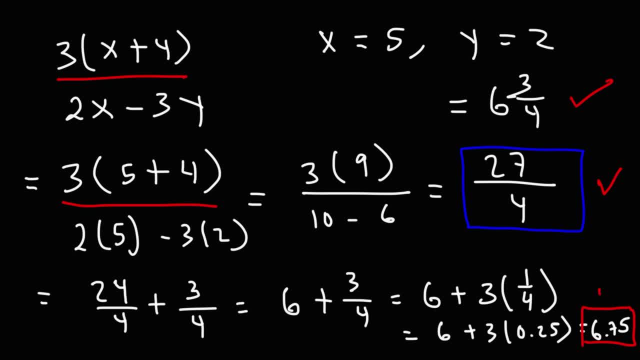 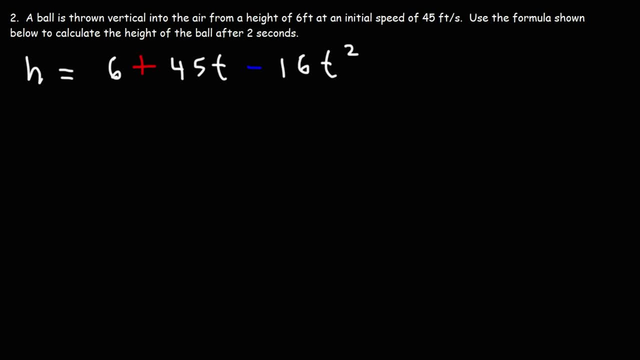 you can leave it as a mixed fraction- 6 and 3 fourths, or as a decimal value: 6.75. now let's put this into application. a ball is thrown vertically into the air from a height of 6 feet at an initial speed of 45 feet per second. 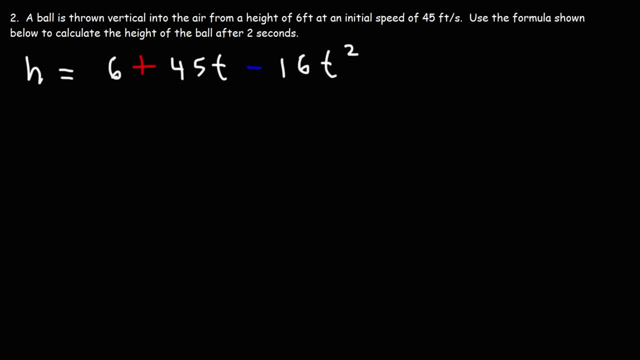 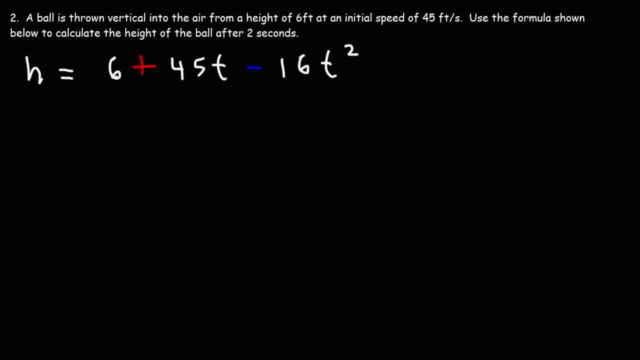 after two seconds. so the height is in the unit, for the height is going to be feet and the time is in seconds. so we have an algebraic expression that relates the height of the ball at any time: t. so to evaluate this algebraic expression, we just got to plug in 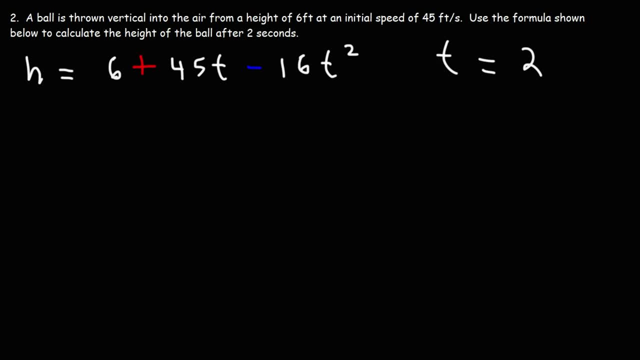 and we're given that t, and we're given that t is equal to two seconds. so let's plug in t into the formula. to get the height, all we need to do is replace t with 2. 45 times 2 is 90: 2 squared, or 2 times 2. 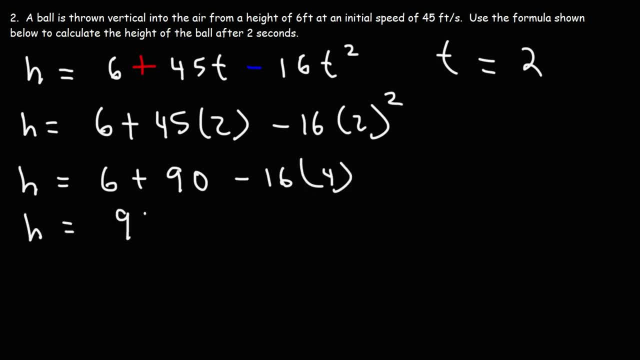 that's going to be 4. 6 plus 90 is 96 and 16 times 4 is 64. 96 minus 64 is 32, so the answer is going to be 32 feet. that's how high the ball will be in the air. 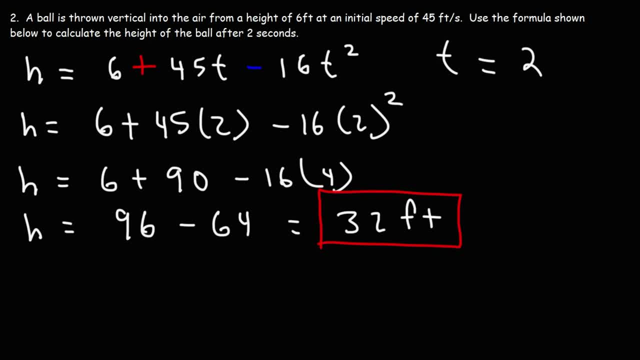 after two seconds. now remember to check your work. plug this portion in the calculator. exactly the way you see it. you should get the same answer. so now you know how to evaluate algebraic expressions. so now you know how to evaluate algebraic expressions. so now you know how to evaluate algebraic expressions.